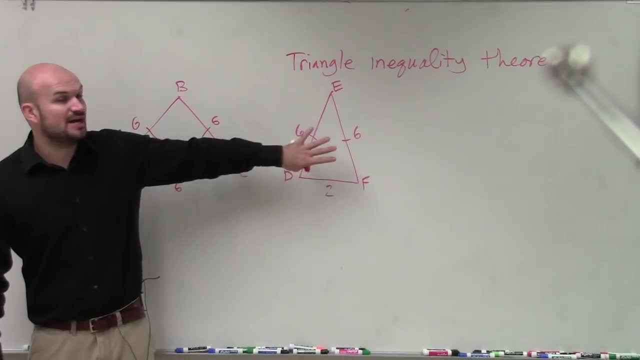 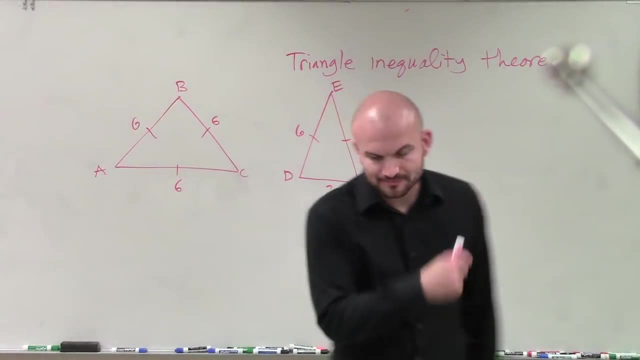 equal. And also what we just again reviewed: when you have an isosceles triangle, your opposite angles are equal. right? That's what we talked about last class as a review. So, anyways, what I want you guys to notice is- or let's maybe. 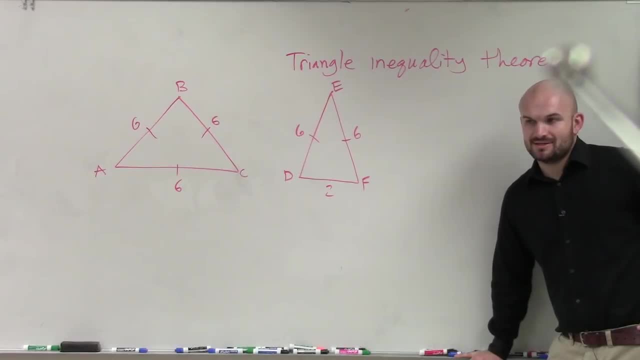 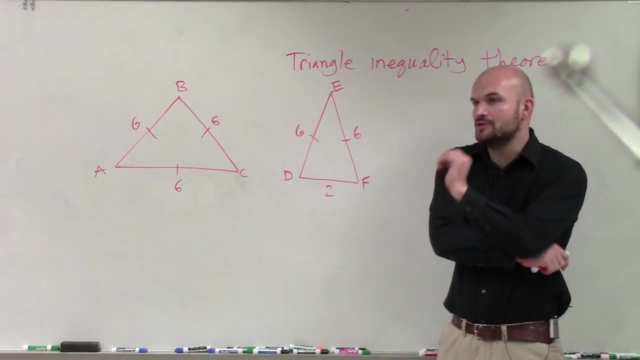 ask you- I'll ask Berta Berta- if I was to add- let's talk about this triangle for right now- If I was to add two sides and compare it to a third side, how would the measure of the sum compare to the third side? 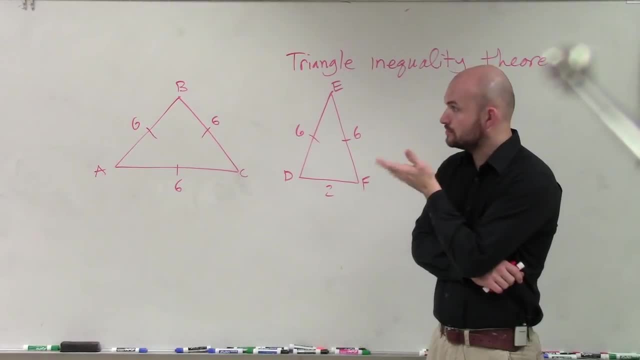 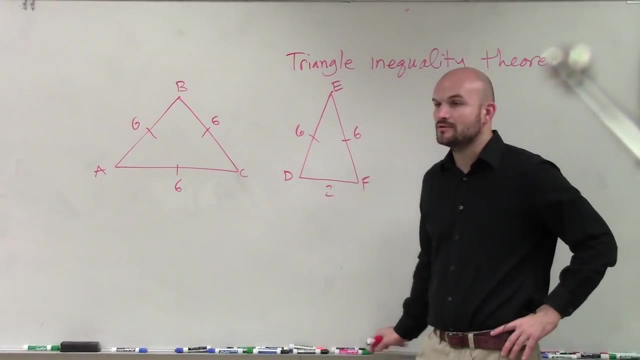 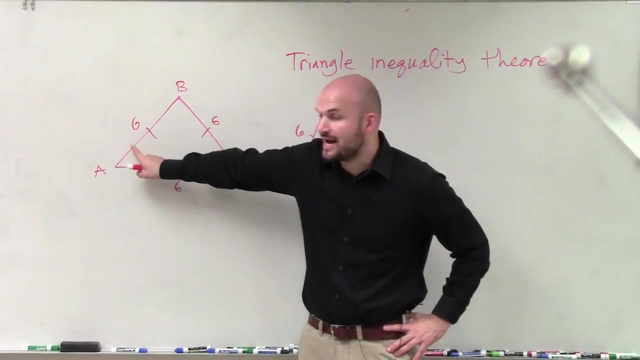 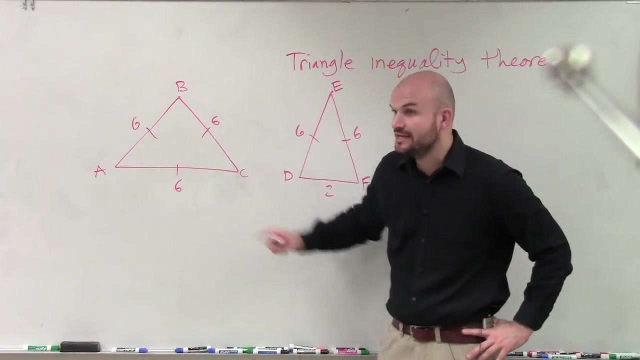 What do you mean? I don't know. Let's do it, Do it in your head. Let's compare this side plus that side and compare it to that side. What would you say now for those two sides? Right, You would say: the addition of AB plus BC, the sum of AB and BC. 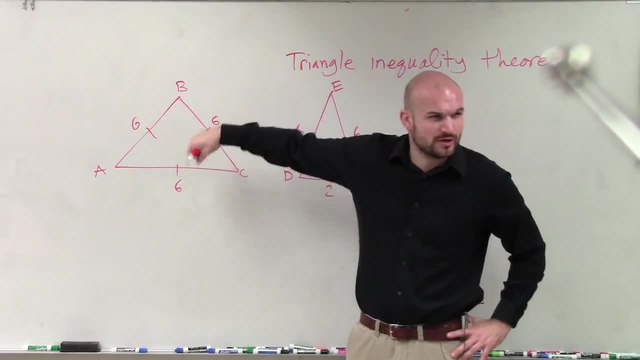 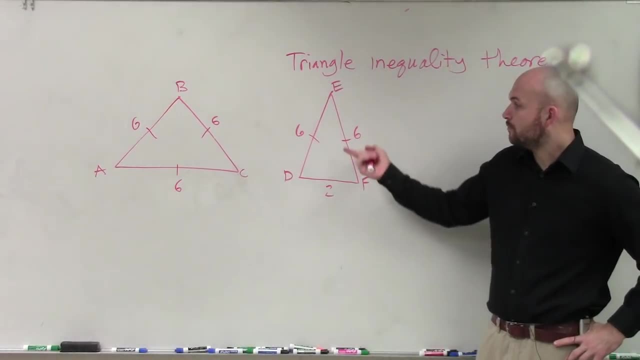 is greater than AC, correct, And would that work for no matter what two sides I choose? Yes, OK, Let's go and look over here, All right, Would? if I take the sum of any two sides, is it always going to be larger than the third side? 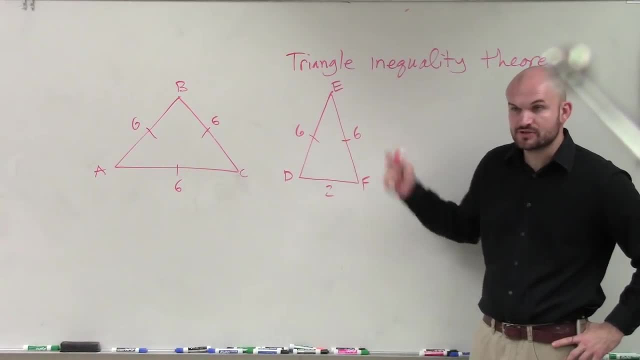 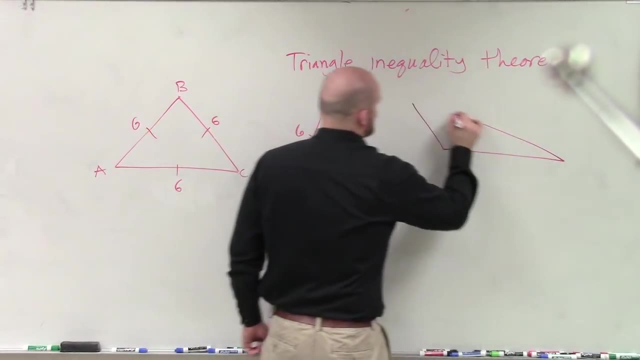 Yeah right, Six plus six is obviously greater. We're in 12.. Six plus two is obviously greater than eight. So we have an equilateral, We have an isosceles. Now let's talk about a scalene. 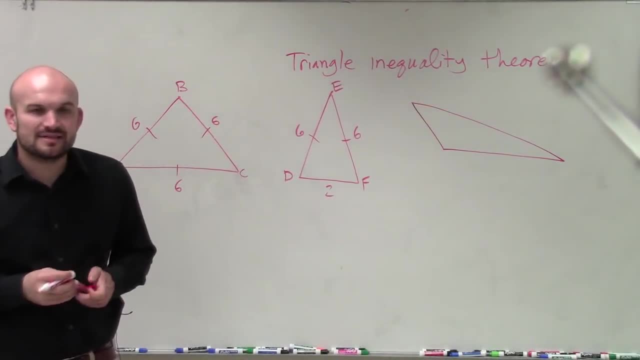 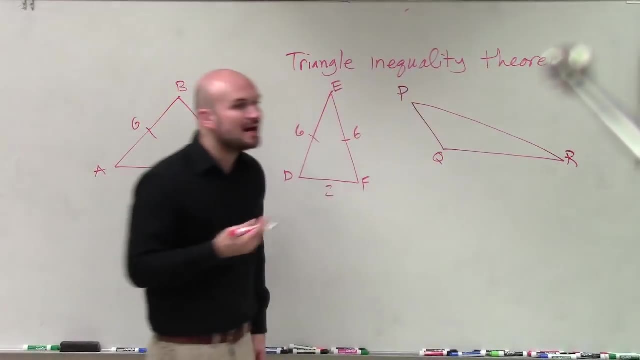 So is that always going to work for a scalene? And, Zach, the answer to that is yes, it does All right. So what we're going to do is say PQR If you guys have a triangle or if you're. 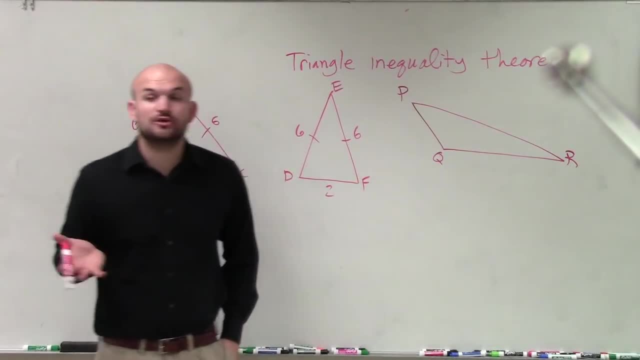 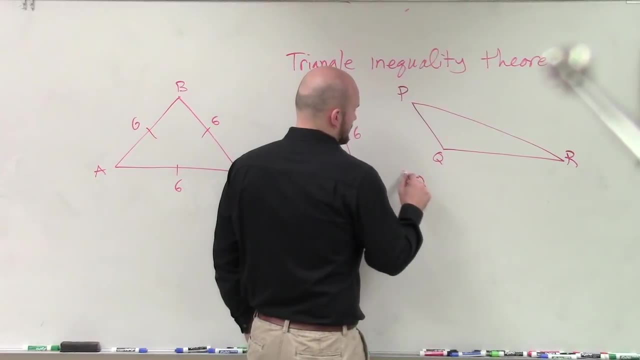 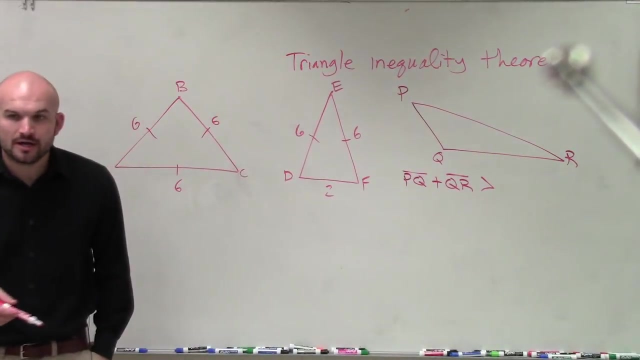 given the sides of a triangle. you want to determine if it will prove to be a triangle. Zach, you're not correcting what I was asking you to do. Then you can take the sum of any two sides, and that has to be greater than the third side. 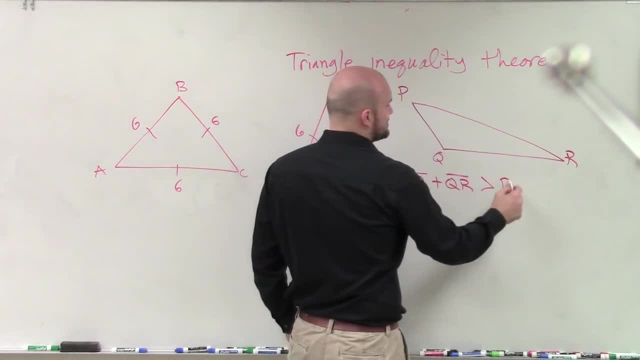 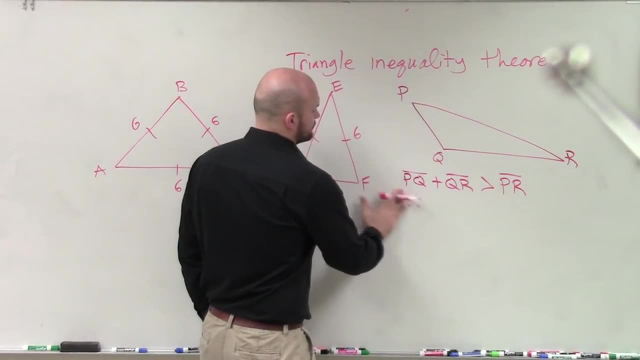 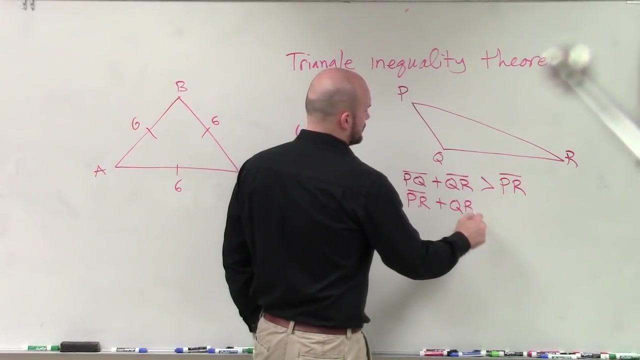 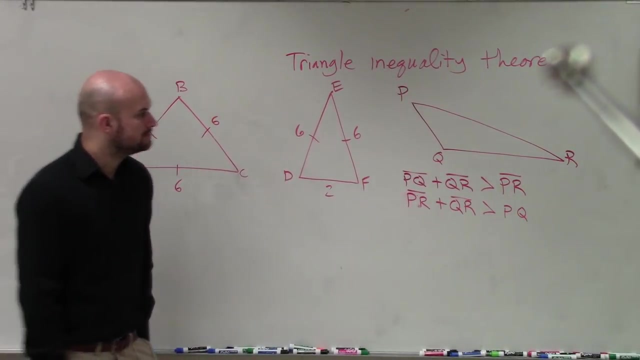 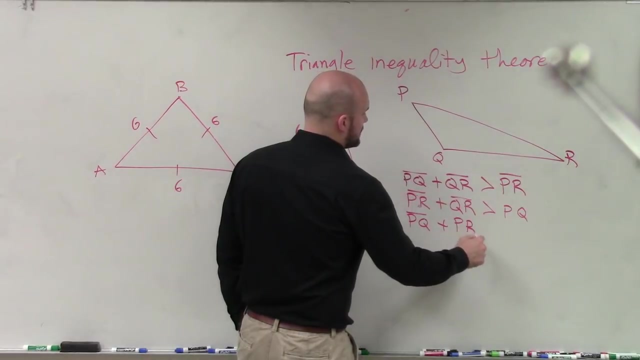 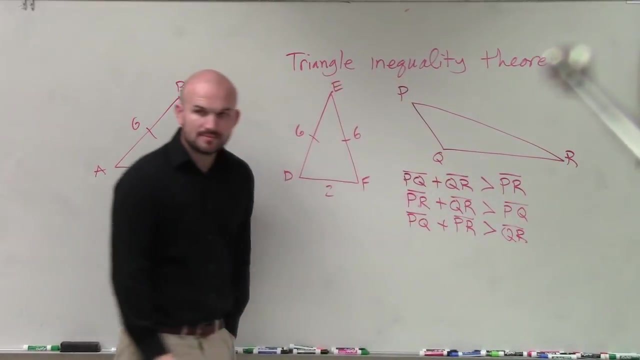 So in this case I do PQ plus QR, That has to be greater than PR. And if I take line PR plus QR, That has to be greater than PQ. all right, And then if I take PQ plus PR, That has to be greater than QR, OK. 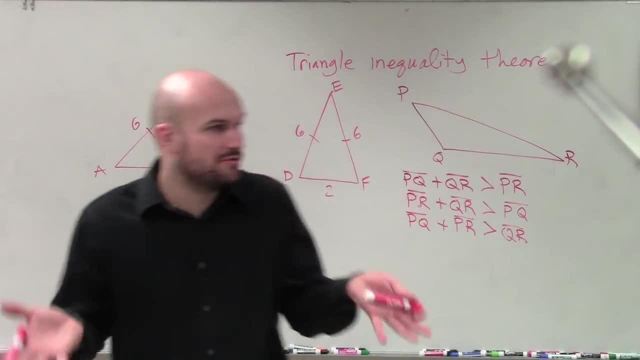 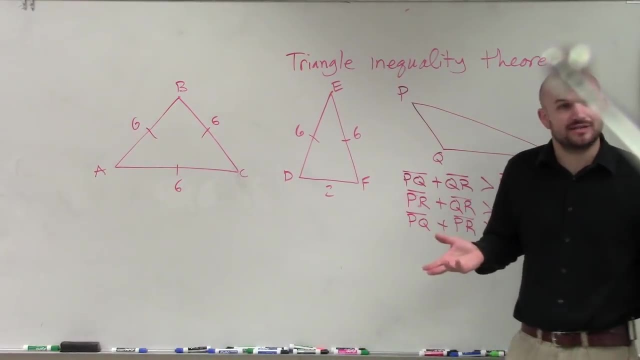 So it's a pretty simple theorem. All it really states, guys, if I give you three sides and I say, is this a triangle? to determine if it's a triangle you just need to take the sum of any two sides and make sure that any two sides are going. 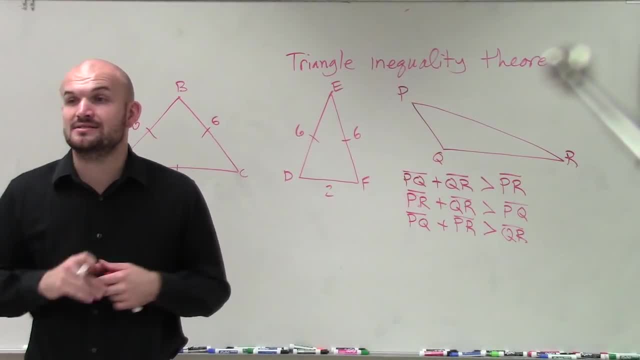 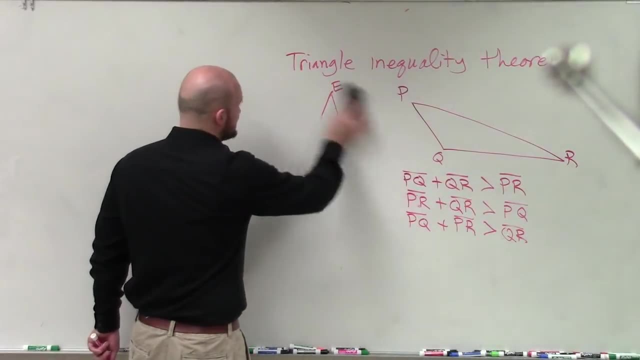 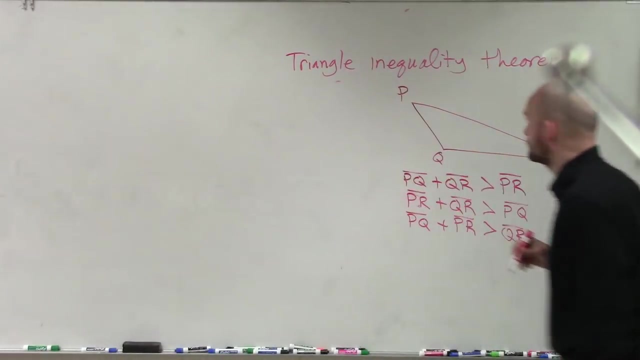 to be greater than the next. Not equal to they have to be greater than. yes, Let's go over two examples. So let's say I give you two side lengths. How do you know automatically what is a triangle? How do you know that? 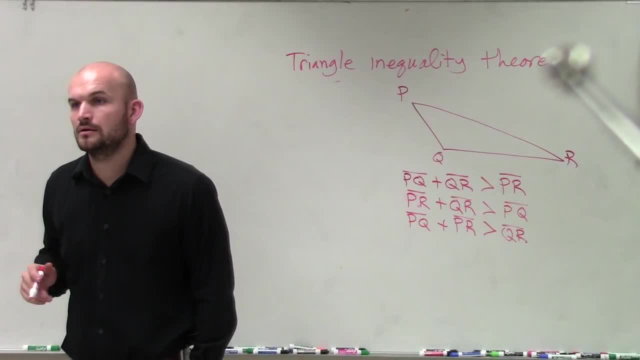 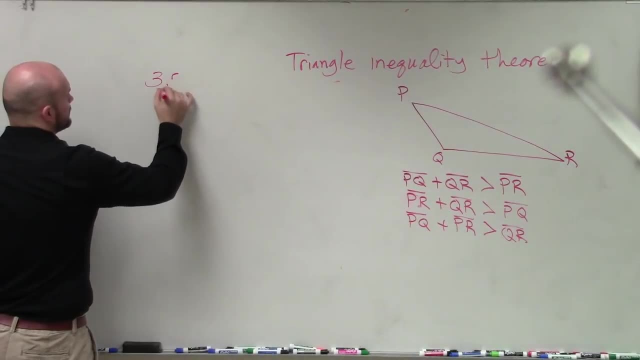 What do you mean? Like, can you just do it? Huh, How do you like? Let me give you two examples. Let me give you an example. OK, How about if I gave you 3,, 5, and 7,? OK, 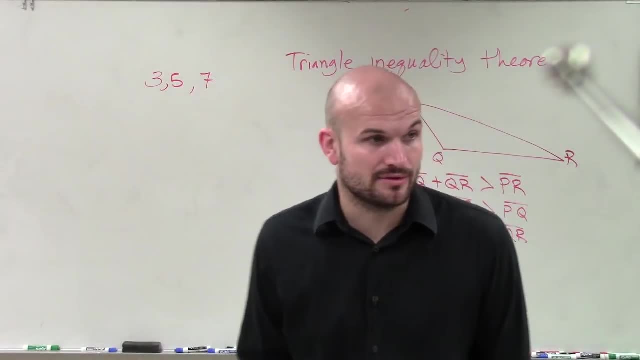 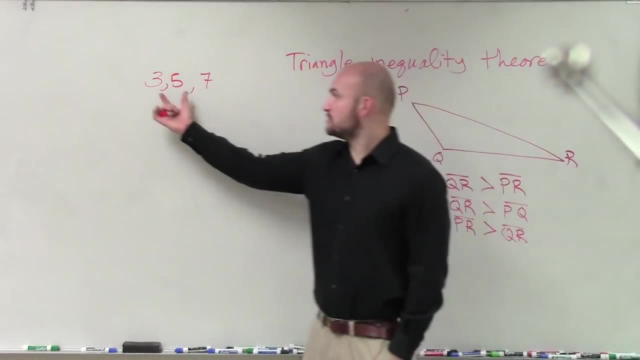 Now remember, if I said, hey, is 3,, 5, and 7,, is that a triangle? What you'd have to do is add up two of the sides and make sure it's greater than the third side. So is 3 plus 5 greater than 7?? 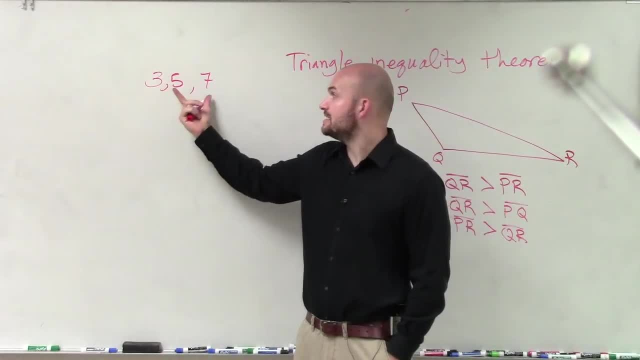 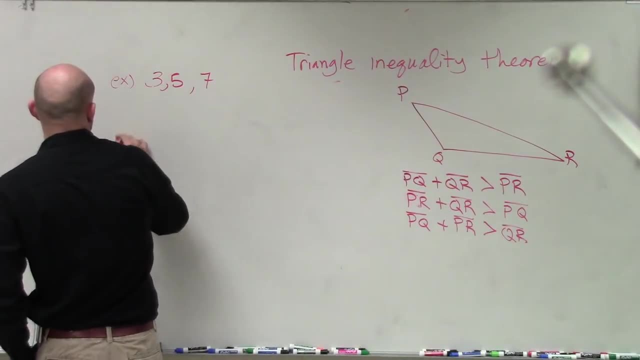 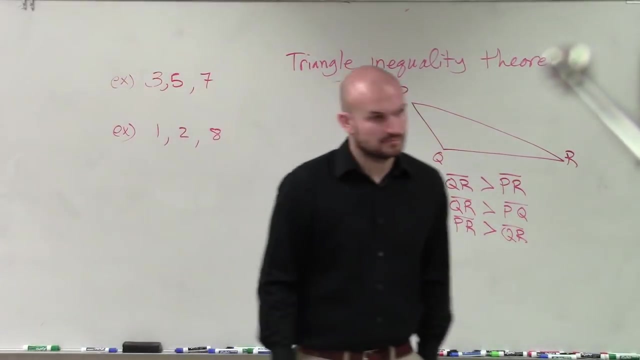 Yes, Is 5 plus 7 greater than 3?? Yes, Is 7 plus 3 greater than 5? Yes, So that's a triangle, right? So let's do one. Let's do maybe a non-example. So what if I did you 1,, 2, and 8?? 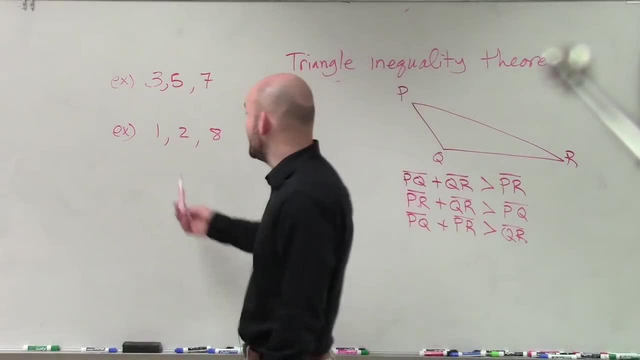 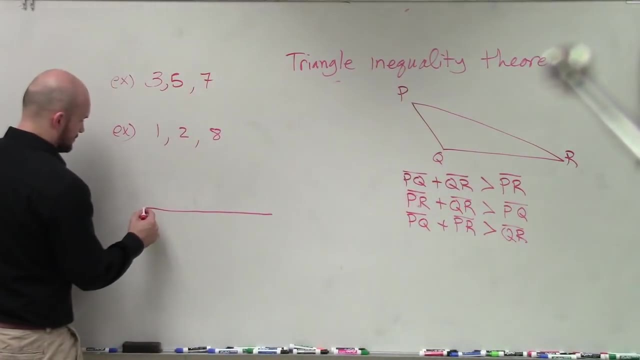 Does that produce a triangle? No, because you can easily say that 1 plus 2 does not equal 8.. And the reason being is- I'm not going to get exact here- Does it have to be greater than or equal? Yeah, it has to be greater than. 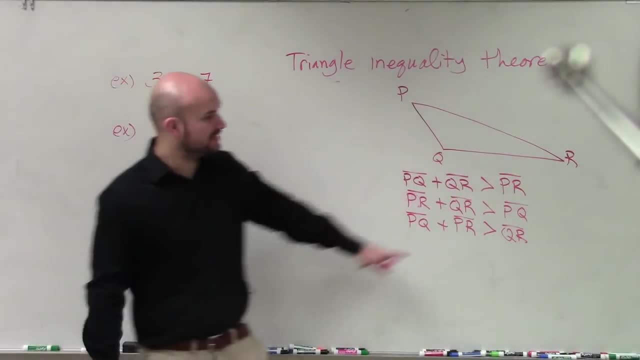 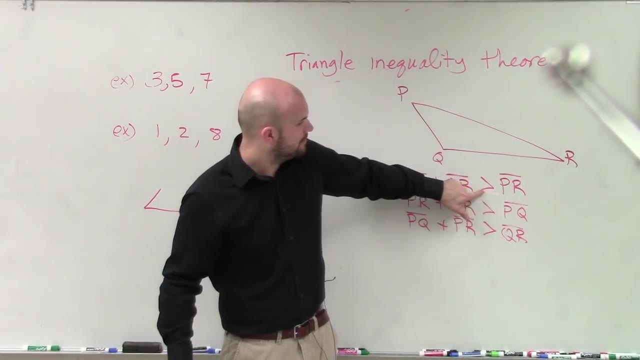 Does it have to be greater or it can't be equal, It has to be greater. There is no equal, Sorry. It has to be greater than There's no equal in here. It's always greater than So in this case, what you guys can see is look at.